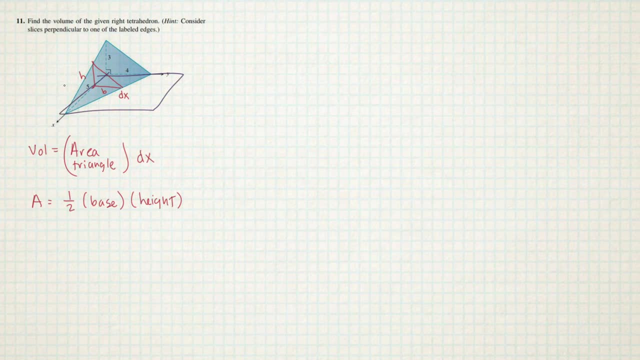 that's going to let me figure out a formula for b in terms of x. All right, so here's the x-axis and here's the y-axis, And we get this kind of line right here, And then, according to the diagram, this distance is 5 and that distance is 4.. And here's our little slice right there: dx. 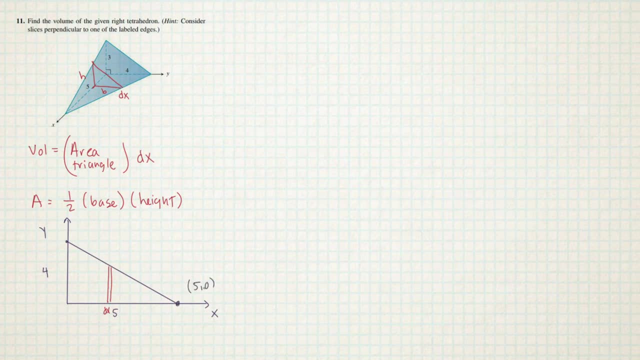 And so that means that this point right here is the point 5, 0.. And then over here I have the point 0.04.. Okay, so obviously this line has negative slope And it's going to be the rise over the run. 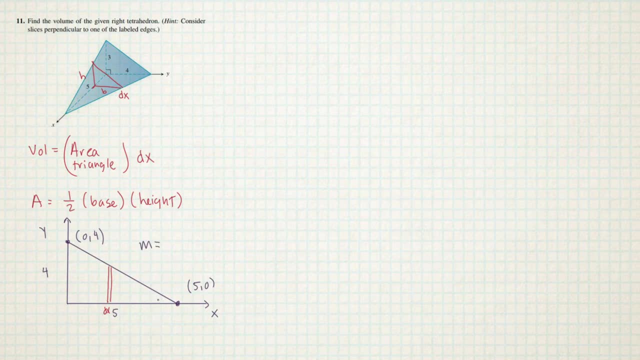 So when I look at this line, I see a slope of negative four-fifths right, The rise over the run. Okay, and also I can just read the y-intercept: off right, there is 0.04.. So that's it, I'm done. 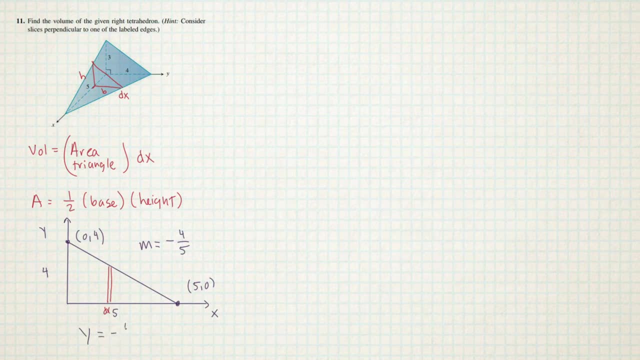 right. The equation of this line is going to be: y is negative, 4, 4-fifths x plus 4.. Okay, sweet. So what that means is, for each fixed value of x, this distance right here is given by that equation, And if we follow this, 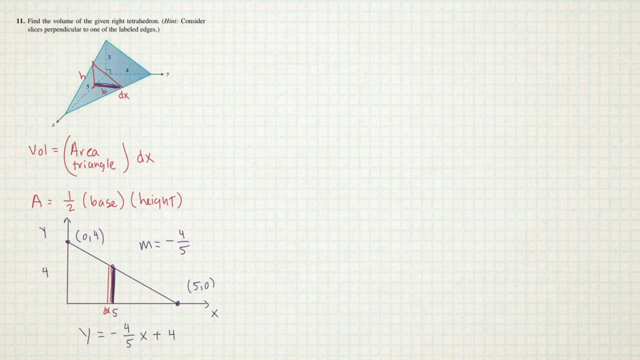 blue line back to the original picture. that's this distance right there. So what that means is that the base is going to be in terms of x negative 4-fifths, x plus 4.. Okay, so now all I need to do is figure out what the height is, So I'm going to go ahead and just 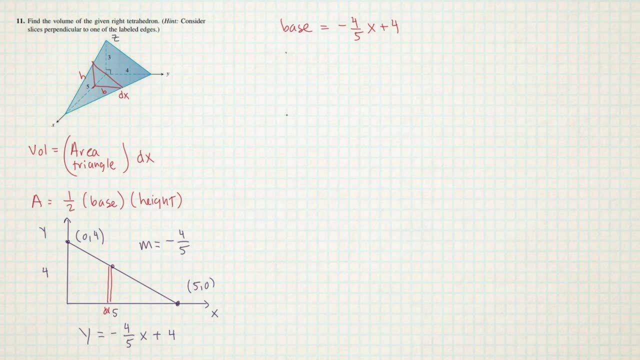 label this axis, the z-axis, And then I can look at this picture in the y, in the x-z plane. So I'm just looking at just this piece of information right here. Okay, so again I get a line, but this: 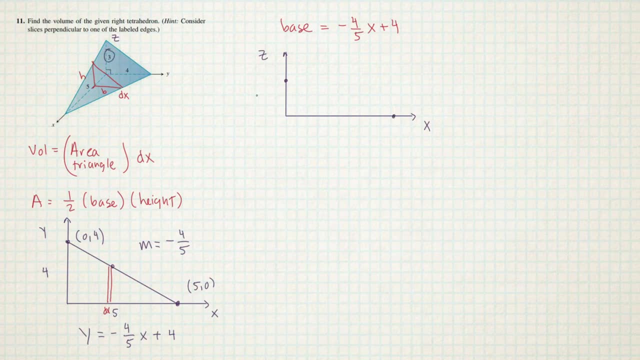 time it's a little bit more shallow right, Because, according to the diagram, the height right here is 3.. and then this distance is still 5. so, as before, I have some small slice right here, dx, and then this point is going to be the 0.50 and that point right there is going to be the 0.03. 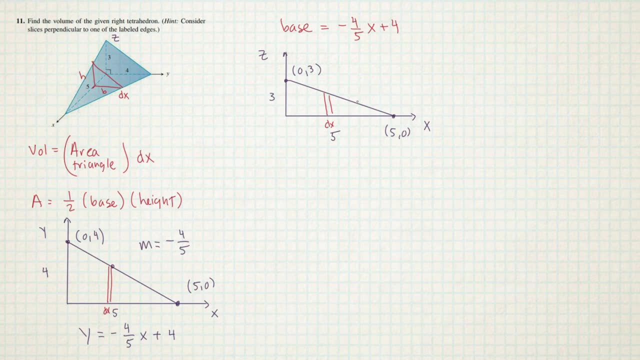 okay, so now I can write the equation of this line. so that means this line here is: obviously, the slope is negative and it's going to be the rise over the run. and then the y-intercept: there is 3. fantastic, so that means that the height of this triangle, right, if we trace this line back. 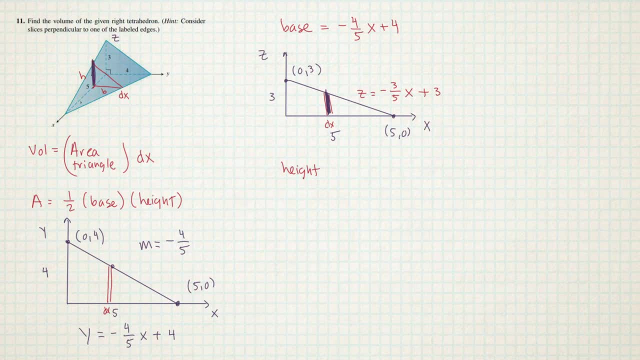 it goes right there on the original picture. so that means the height of this triangle in terms of x is negative: three-fifths x plus 3. so that's it. that means that the area is going to be one-half times the base. that's the height of this triangle. right, if we trace this line back, it goes right there on the original. 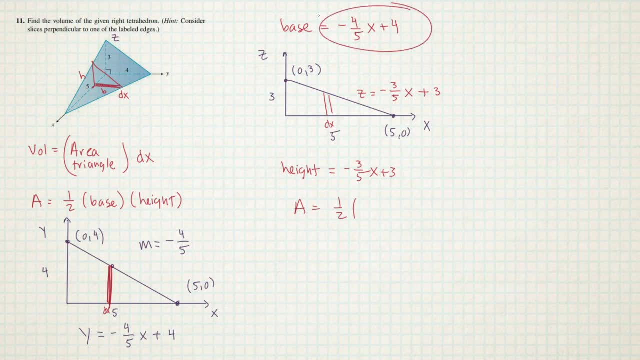 this distance right here and that's that distance right there which we worked out to be this formula. So what is it? Negative, four fifths x plus four. And the height is what we just worked out in terms of z, z and x. So, negative, three fifths x plus three, Awesome. So now we need to. 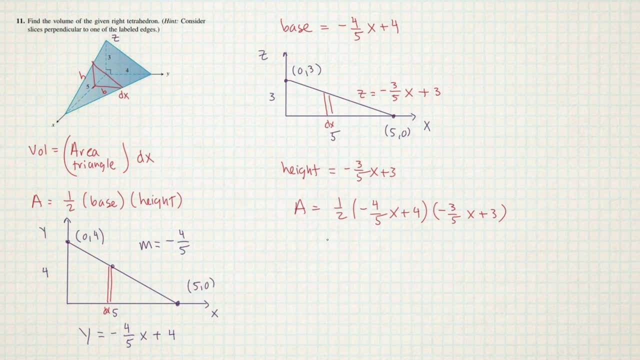 do here is set up the final integral. So we've sliced this perpendicular to the x-axis. So that means x is the variable integration here. So the total volume of this tetrahedron is going to be some integral in terms of x. So which x's give us a triangle. that's in the picture I mean. 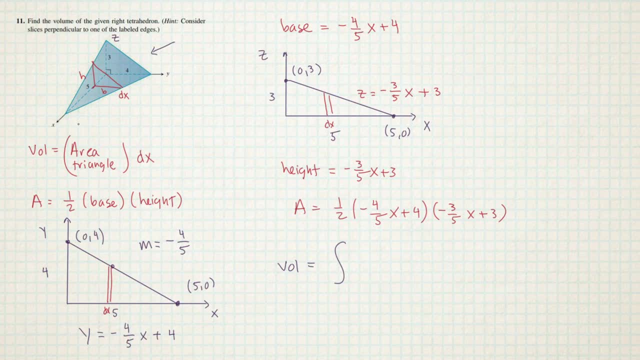 obviously, if I pick some x over there, then that triangle is not going to be in the picture, And if I pick some x over there, that triangle is not going to be inside the picture. So all the x's that we care about are going to be in the picture, So we're going to have a triangle. that's in the 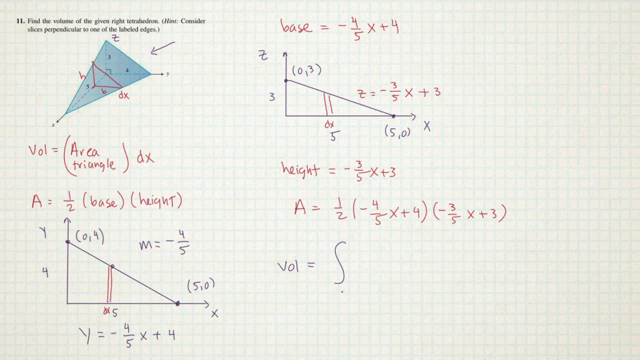 about. here are these x's right here? those are the x's between 0 and 5. so x is going to go from 0 up to 5, and then the formula for the area of each one of these pieces. so that's the base, and then 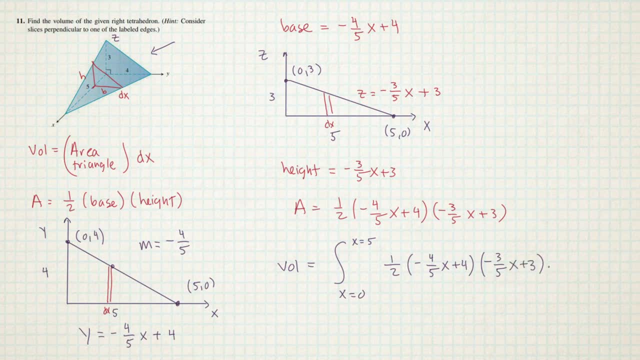 here's the height, and then you got to multiply by the thickness, so that's dx. so that's it. so work out that integral and that'll give you the total volume of this tetrahedron. let me know if you have questions.